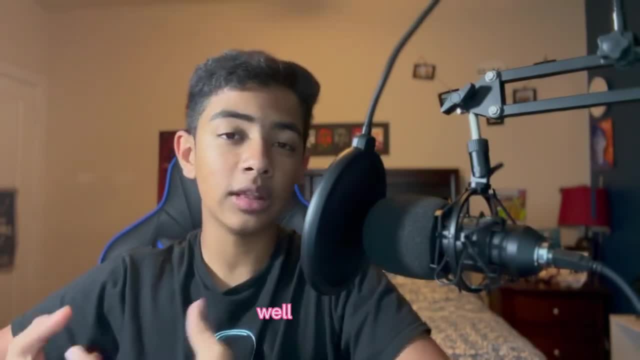 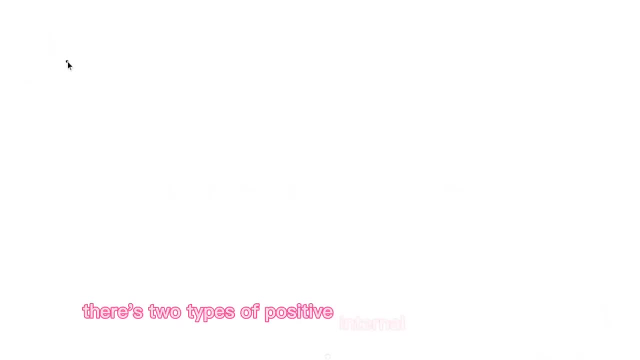 Has a problem like this ever stopped you in your tracks before? Well, in this video we're going over positive integral divisors, so let's do it Alright. so there's two types of positive integral divisor problems. There's the total amount of positive integral divisors and then there's the sum of all positive integral divisors. 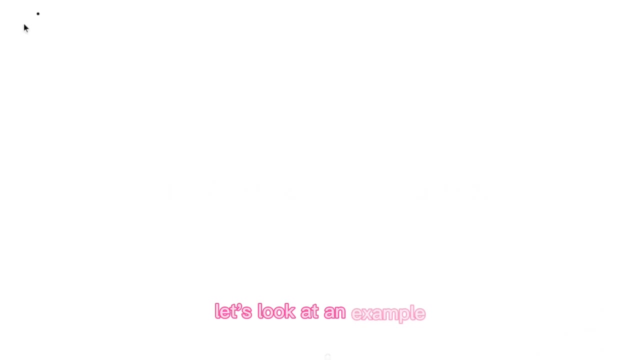 So to solve both we need to know how to, And for that let's look at an example. So let's take the number 36.. Alright, so the total number of positive integral divisors. So we need to know the prime factorization. So in this case, 36.. So the prime factorization? 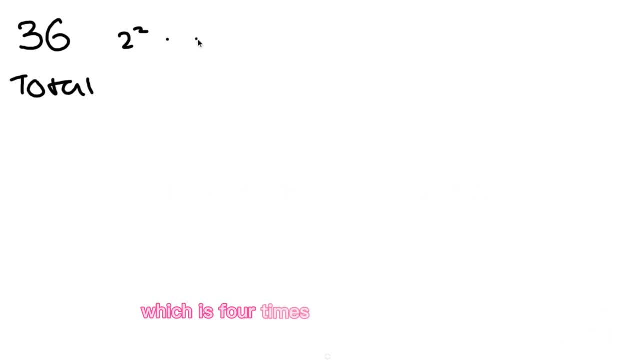 is two squared, which is four times three squared, which is nine. So two squared times three squared is a prime factorization. So now we take these exponents, So we have two as the first exponent and two as a second exponent, and we're going to add one to each. 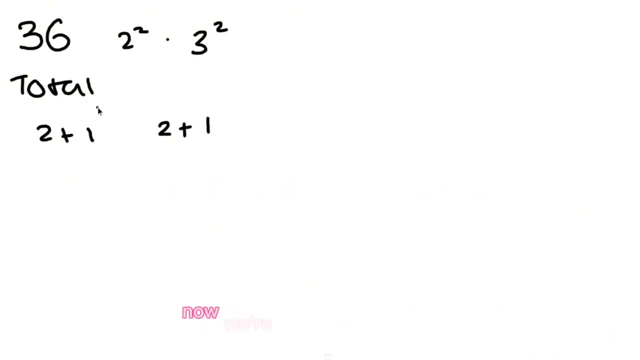 of them. So two plus one. two plus one, That's just three and three. Now we're going to multiply them. So two plus one times two plus one, That's just three times three, and that's three, that equals 9.. So that's the total amount of positive integral divisors. Now let's 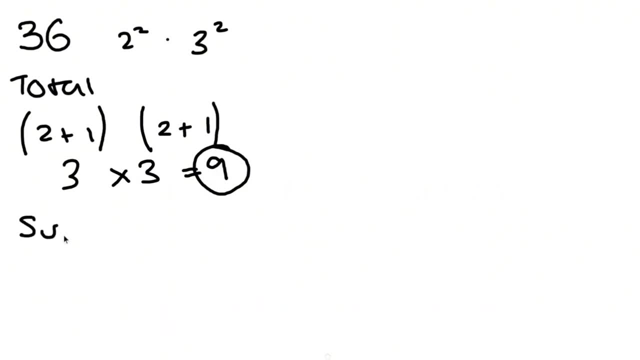 know how to solve the sum of all positive integral divisors. So we need to look at the prime factorization again. So we have 2 squared and we have 3 squared, Alright. so we first need to raise the power by 1.. So 2 squared becomes 2 cubed and 3 squared becomes 3 cubed. 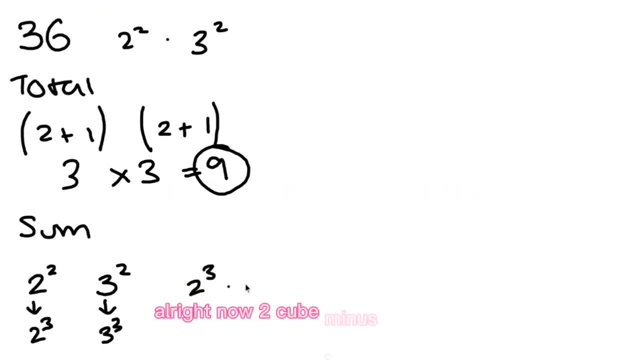 Alright now 2 cubed minus 1 over 2 minus 1.. And now we multiply that times 3 cubed minus 1 divided by 3 minus 1.. Alright, so 2 cubed minus 1, that's just 8 minus 1, which. 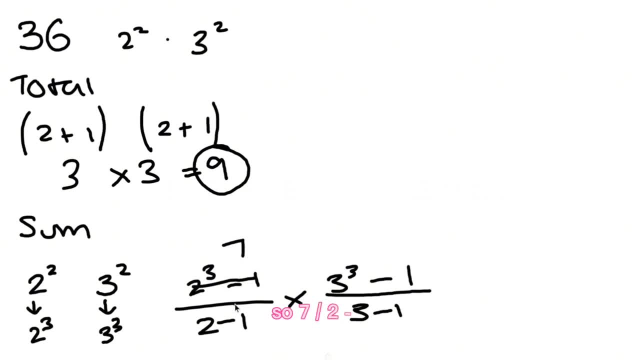 is 7.. So 7 divided by 2 minus 1.. 2 minus 1 is just 1.. So it's 7 over 2 cubed minus 1.. So 7 over 2 cubed minus 1 is 1, which is 7.. So 7 multiplied by 3 squared minus 1, which. 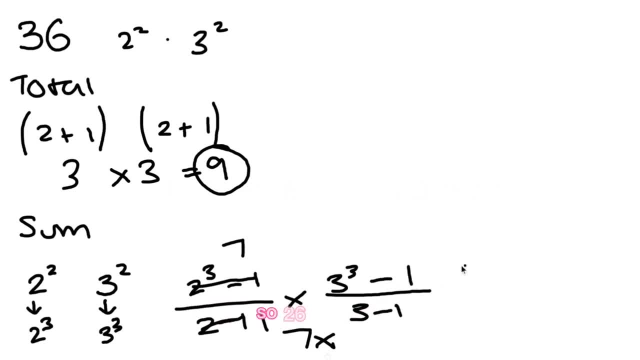 is 26, divided by 3 minus 1,, which is 2.. So 26 divided by 2 is 13.. So now we have 7 times 13,, and that equals 91. And that's your answer, Alright, first, what is the sum of all the? 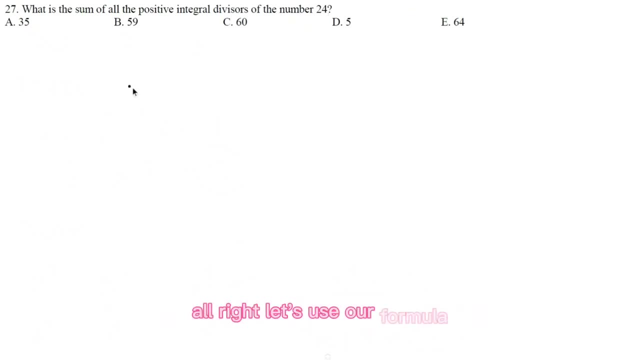 positive integral divisors of the number 24?? Alright, let's use our formula. So we first need to know the prime factorization of 24.. So 24 can be broken down by the number 24.. So 24 can be broken down by the number 24.. So 24 can be broken down by the number 24.. 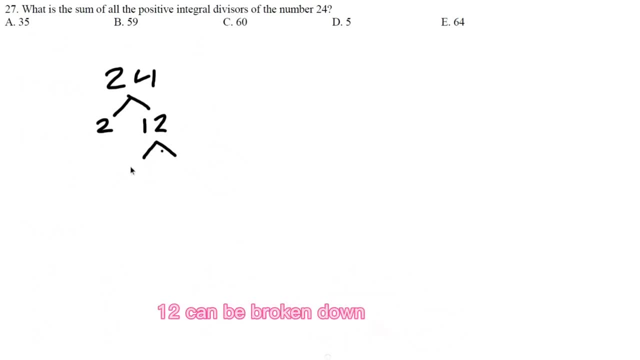 So it can be broken down by 2 and 12.. 12 can be broken down by 6 and 2. And 6 can be broken down by 3 and 2.. Alright, now we can't divide it anymore, So we take up the first. 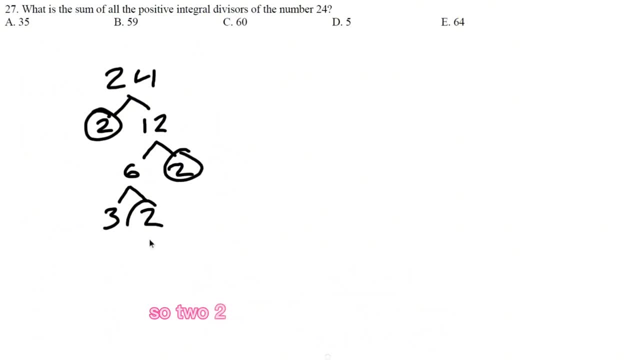 number, which is 2.. So 2, 2, 2.. So 2 comes three times, which means the first number is 2 cubed, Next we have 3.. So 3.. 3 only comes once, so it's just 2 cubed times 3.. 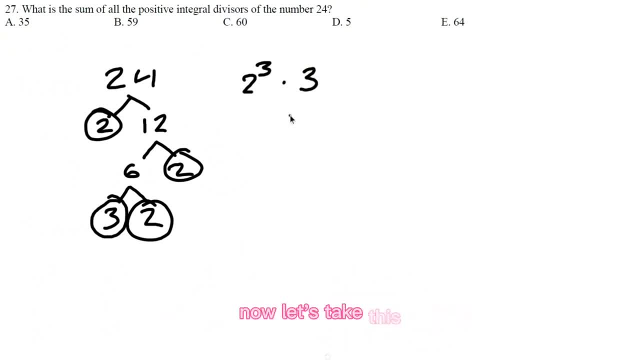 So that's the prime factorization. Alright, now let's take this and solve for the sum of all positive material divisors. So we need to raise the powers by one, so this becomes two power four and three power two. Now we need to put it into the formula. 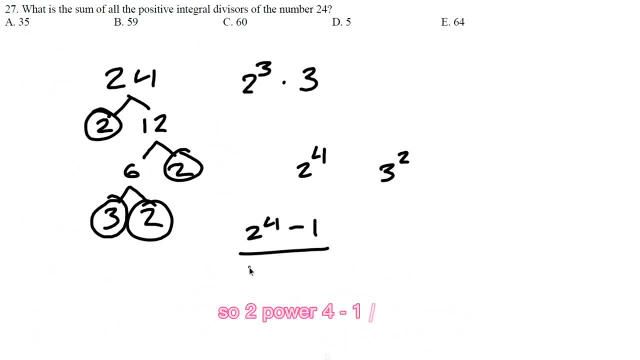 So two power four minus one, divided by two minus one, times three, squared minus one, over three minus one, All right, so two power four is 16, 16 minus one is 15.. So 15 divided by two minus one, which is one. 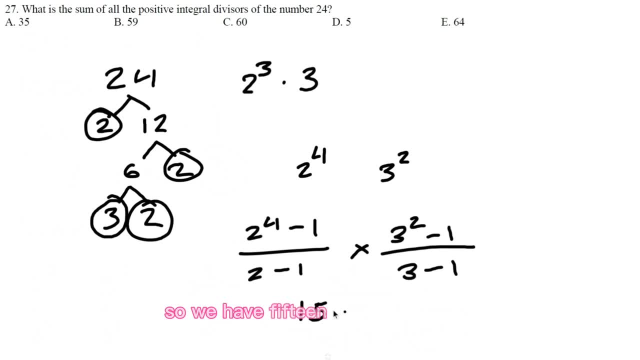 All right, so that's just 15.. So we have 15 times three squared, which is nine. Nine minus one, that's eight. Eight divided by three minus one. Three minus one is two, so eight divided by two. So eight divided by two is four. 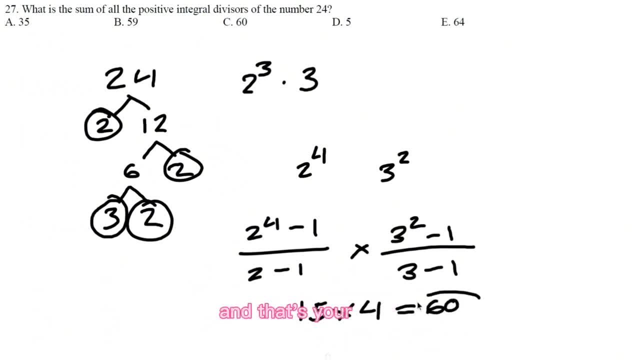 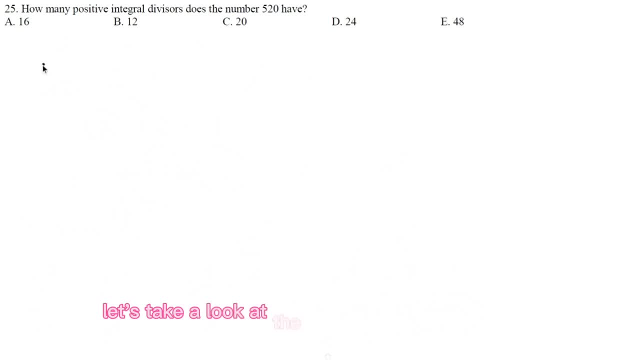 So 15 times four is 60, and that's your answer, All right? next, how many positive integral divisors does the number 520 have? All right, let's take a look at the prime factor in relation to 520. 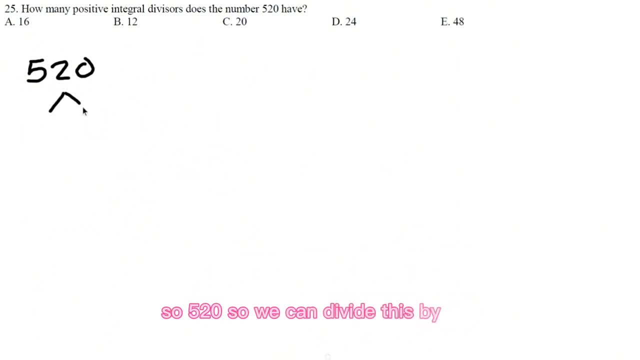 So 520, so we can divide this by two, and that's two and 260.. This can be further divided by two, so two and 130.. This can be further divided by two, two and 65.. 65 can be divided by five, so five and 13.. 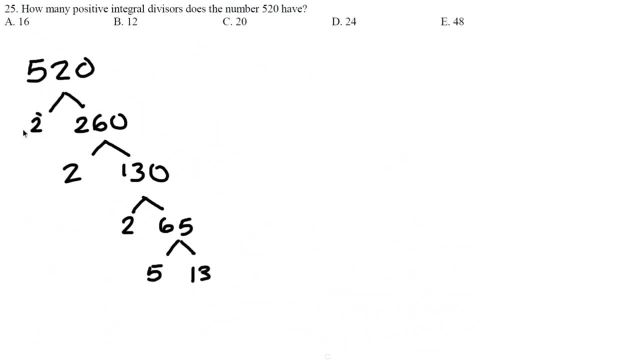 And 13 can be divided by anything, All right. so we have two, two, two. So that's two power three, because there's three twos, We have five ones and we have 13 ones. So two cubed times five times 13.. 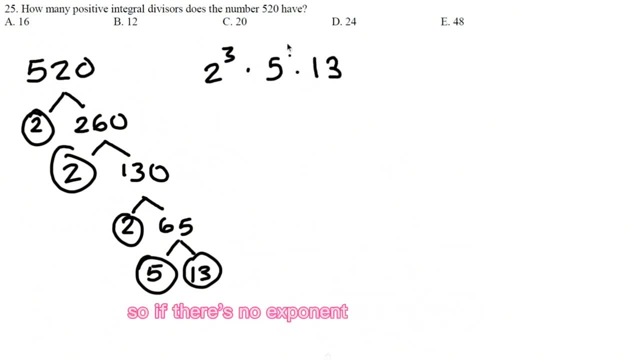 That is a prime factorization, So if there's no exponent above the number, we can just assume that it's to the power of one. All right, so now what we need to do is we need to raise the exponents by one. 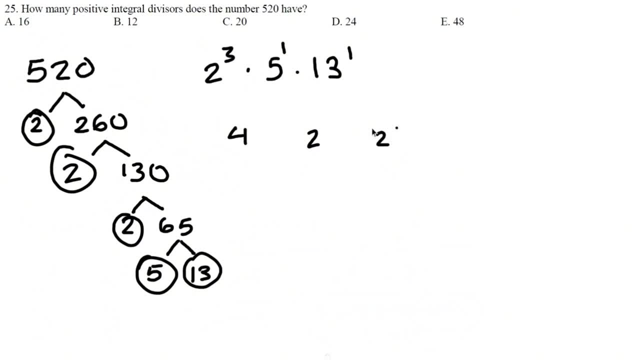 So that's four, two and two, And now we just multiply all these. So four times two is eight, Eight times two is 16.. All right. next, How many positive integral divisors does the number 2,000 have? 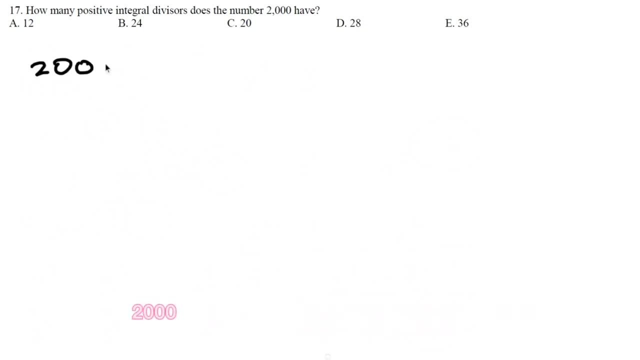 So let's find the prime factorization. 2,000 can be broken up into two and 1,000.. 1,000 can be broken up into two and 500.. 500 can be broken up into five and 100.. 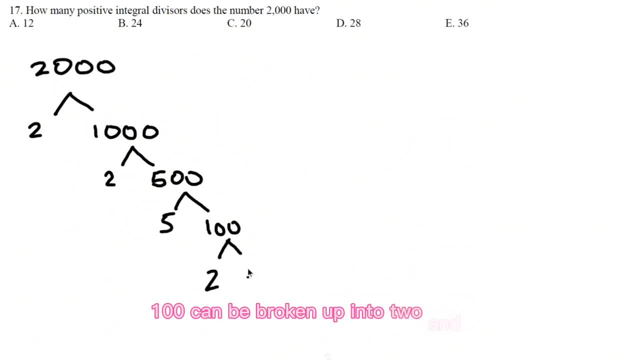 100 can be broken up into two and 50.. 50 can be broken up into five and 10.. And 10 can be broken up into five and two. All right, let's start off with two. So we have two, two, two and two. 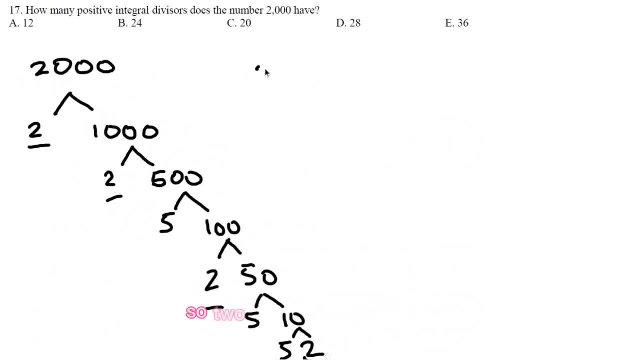 All right, so that's one, two, three, four, two, So two power four times one. two, three, So that's three, fives, So that's five power three. So we take our exponents, which is four and three. 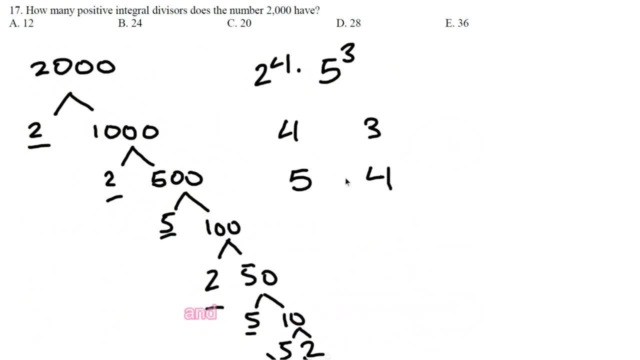 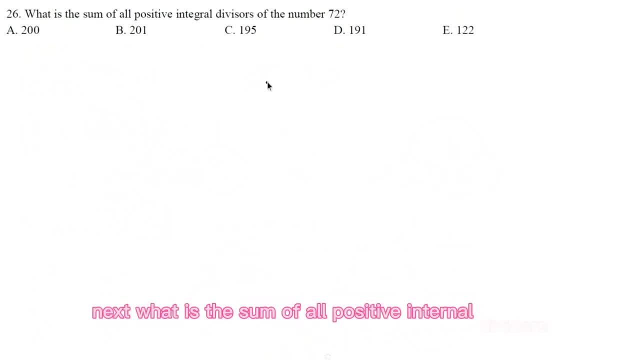 and we need to raise them one, So that becomes five and four, And then we just multiply them. So five times four equals 20, and that's your answer. Next, what is the sum of all positive integral divisors of the number 72?? 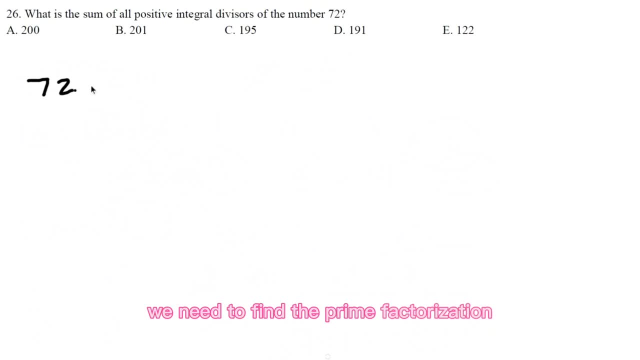 All right. so if we look at 72, we need to find the prime factorization. So 72 can be divided by two into two and 36.. 36 can be divided into nine and four, And nine can be divided into three and three. 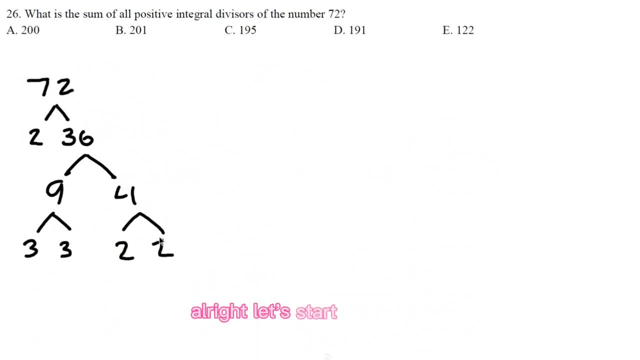 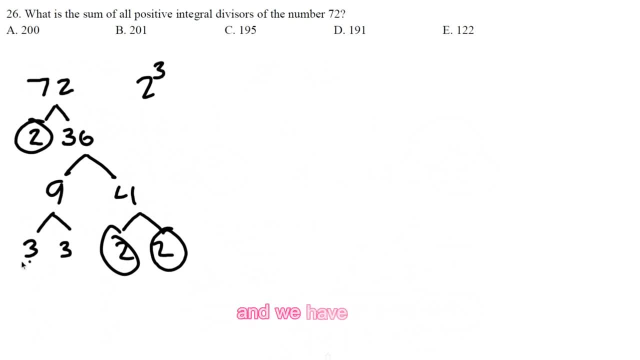 So we have three twos, so that's two power three. And we have one two, So we have two threes, So that's three power two. All right, so now we take the exponents and raise them by one. 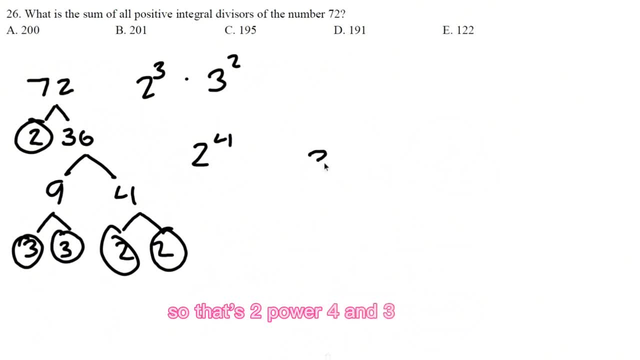 So that's two power four and three power three. Now let's put them into the formula. So two power four minus one over two minus one times three cubed minus one. All right, so this is just one. So two to the power of four is 16.. 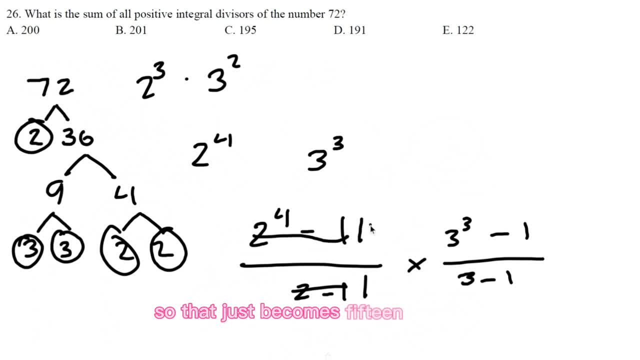 16 minus one is 15.. So that just becomes 15 over one, which is 15.. So 15 times three minus one, that's just two. Then three cubed is 27.. 27 minus one is 26.. 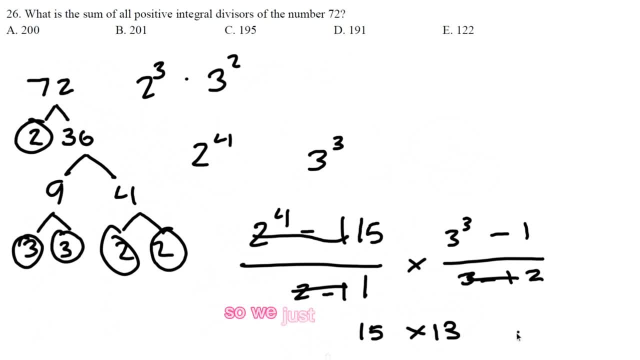 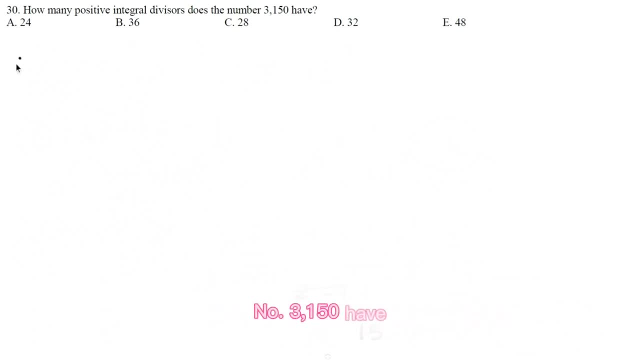 26 divided by two is 13.. So we just do 15 times 13.. 15 times 13 equals 195, and that's your answer. Next, how many positive internal divisors does the number 3,150 have? 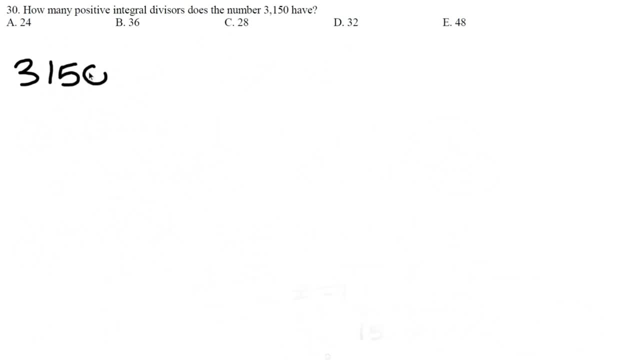 All right, so 3,150.. So this can be divided into five, So five and 630.. 630 can also be divided by five, So five and 126.. This can be divided by two, So two and 63.. 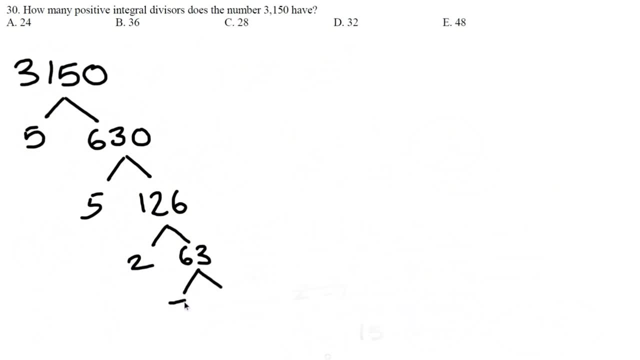 And 63 can be divided by seven and nine, And nine can be divided by three and three. All right, let's start off with two. We have one, two, So just two or three. power one, if you want, Then three. 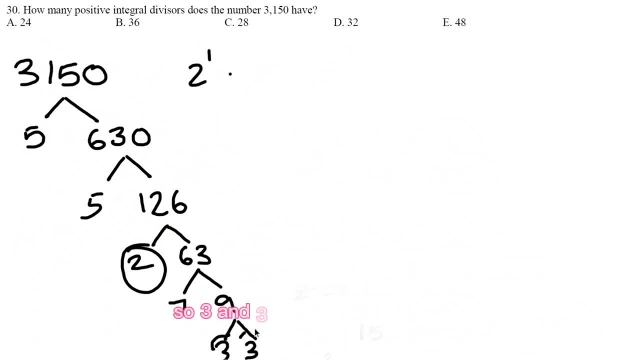 We have three twice, So three and three, So that's three squared. Then five: We have five twice as well, That's five squared. And then we have seven once, So just seven, Or, if you want seven, power one. 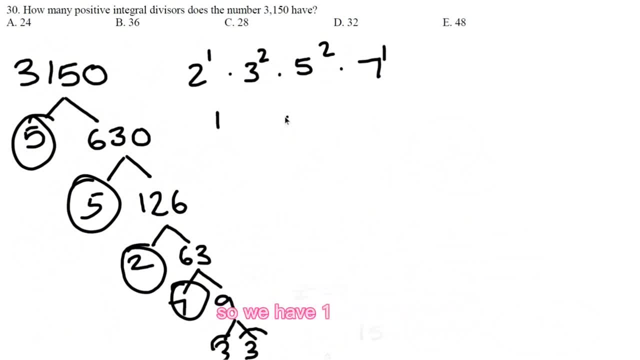 All right, now we take the exponents, So we have one, two, two and one, And we raise them all by one, So this becomes two, three, three and two. Now we just multiply all of these, So that's just six times three times two. 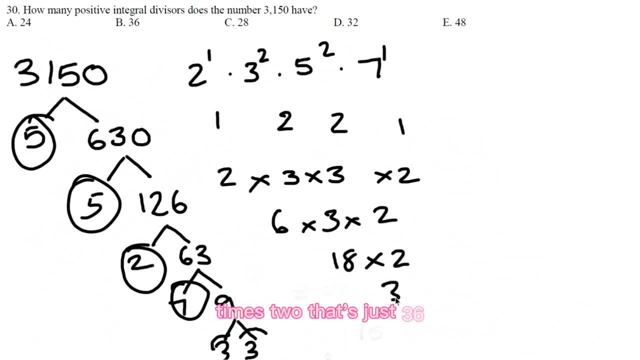 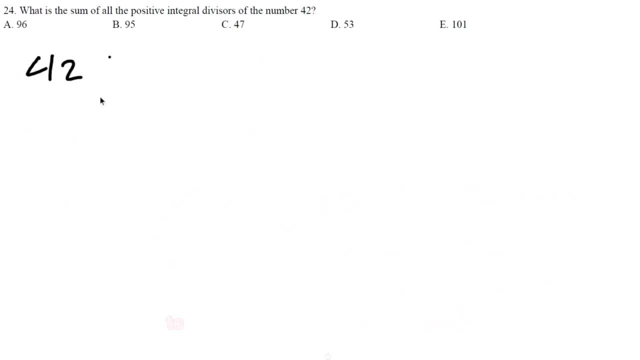 That's just 18 times two, That's just 36.. And that's your answer. All right, what is the sum of all the positive integral dividers of the number 42?? So to find the prime factorization of 42,, we can do this divided by two, or we can divide. 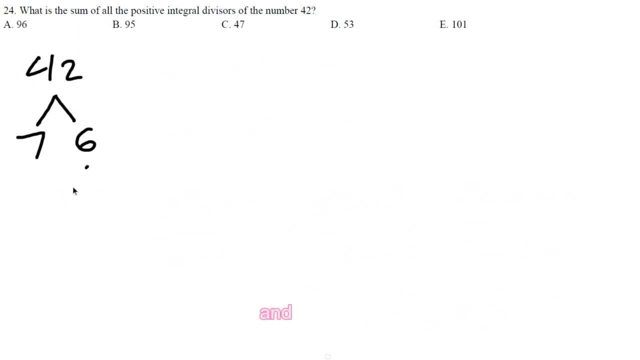 it by seven. So 42 divided by seven is six, and six is three times two. So now we have our three prime factors, so two, three and seven. So, since they only appear once, it's two power one times three power, one times seven power. 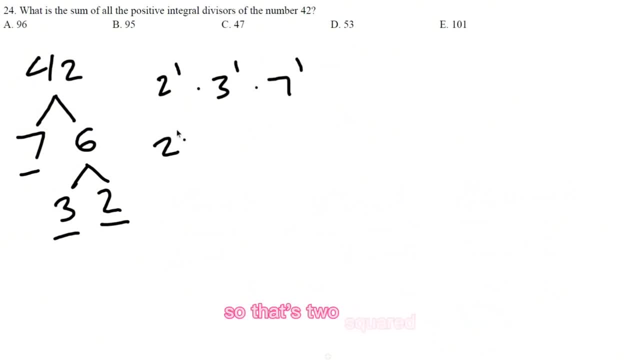 one. All right, now we need to raise all our powers by one. So that's two squared, three squared and seven squared. Now let's put this into the formula. So two squared minus one over two minus one times three squared minus one over three minus. 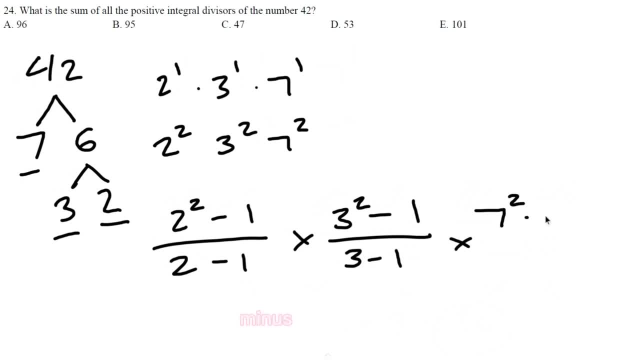 one times seven squared minus one over seven minus one, All right. so let's simplify the denominators. Two minus one is just one. Three minus one is just two. Seven minus one is just six. All right, so we have one, two and six for the denominators. 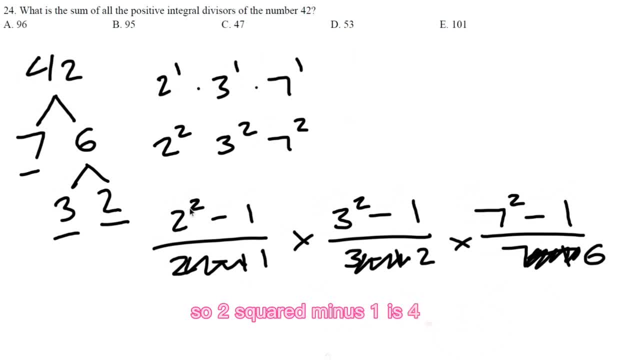 Now let's look at the numerators. So two squared minus one is four minus one, and that's three. Three squared minus one is nine minus one, and that's eight. And seven squared minus one is 49 minus one, and that's 48.. 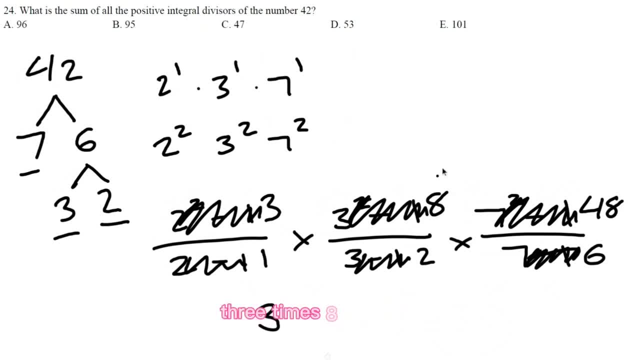 So three over one is three. Three times eight over two. Eight over two is four. Three times four times 48. divided by six, Forty divided by six is eight. All right, so this simplifies to 12 times eight, because three times four is 12, and